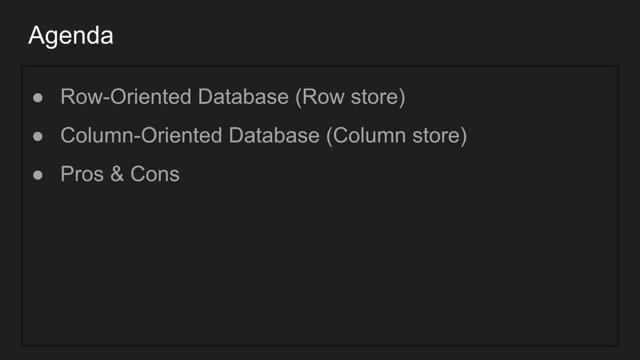 to discuss what is a row-oriented database, or also called row store database, because that's the store type. How is it stored on disk, right? I'm going to also describe the column-oriented database, or also known as column store, or another fancy name is columnar database, because 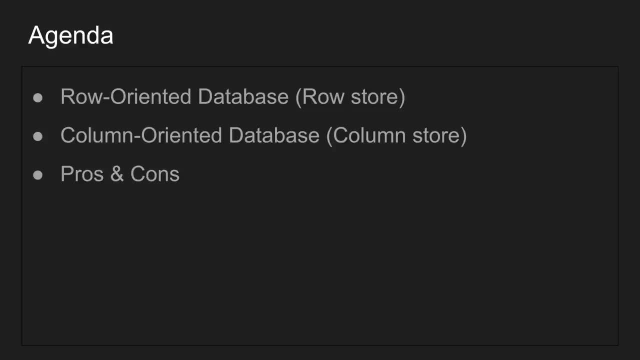 yeah, why not? Just let's confuse everybody by inventing new names. So it's all the same thing. It's just So how things are stored on this. We're going to talk about the difference these two, And then, finally, we're going to discuss pros and cons of both. How about we jump into it, guys? All right, 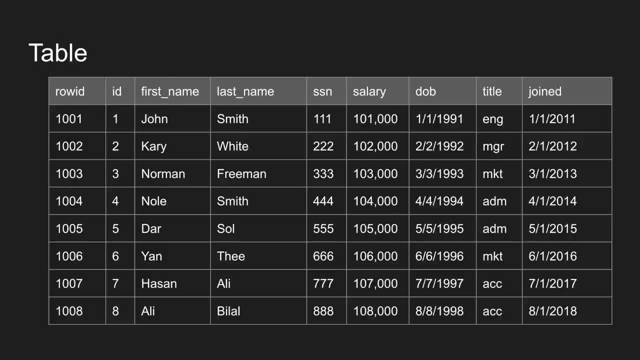 guys. So let's say we have a beautiful table like this. okay, It's an employee's table, It doesn't only have eight rows, It has thousands and thousands of rows, right, But for simplicity, we only have these. These are the columns, straightforward And the first I want you. 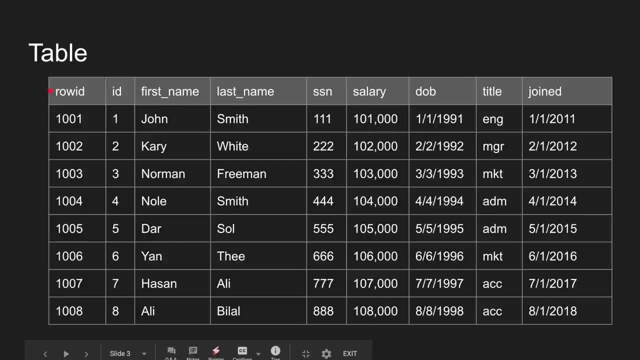 to pay attention to this. This is the row ID. This is how databases. It's a unique identifier that identifies the row. It's different than the primary key or this ID. It's just something that has Most of the time. most databases have this internal mechanism to identify this row. okay. 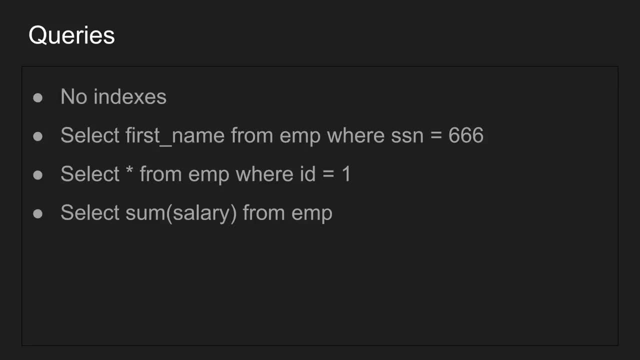 And I want you to pay attention to this. So if I'm going to submit a bunch of queries on this table, I want to do this without any indexes, because indexes will just complicate the manner and by way we think about column versus row, again, I want to take them out of. 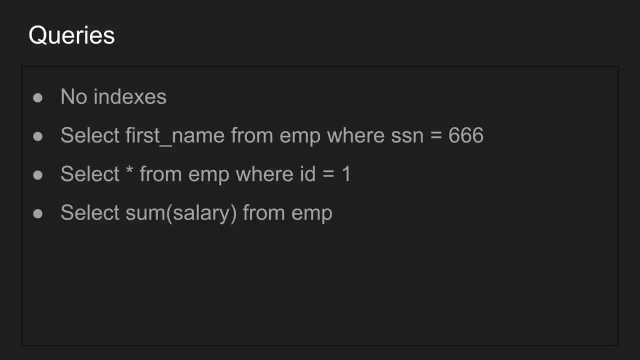 the equation and think about them. just, We don't have any indexes, We're just scanning the table to answer these following questions. So these are the following queries that I'm going to execute on a row database, And then I'm going to execute the same exact queries on column database and see: 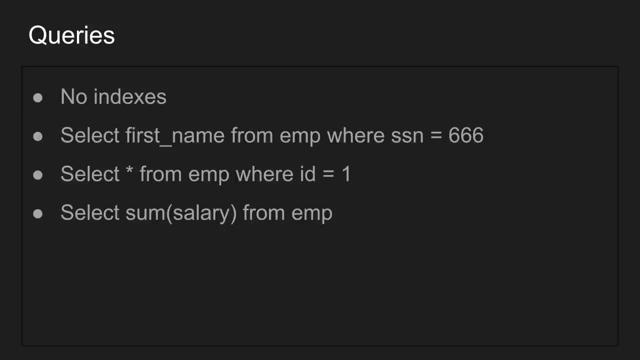 which one does best for each style of how we're going to store these tables. right The same table, we're going to store it on row. The same table, we're going to store it on column storage. And then we're going to look how these queries perform. So select first name from. 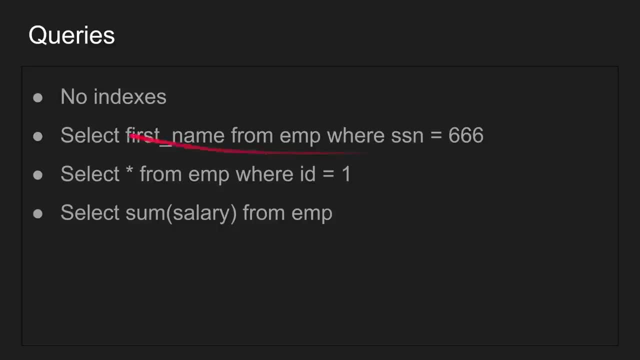 employees where social security number equals 666, the devil. And then we're going to select star from employee where ID equals 1.. Very simple, okay. And the final is to select sum. We're just going to sum all the salaries of the employees, for some reason. 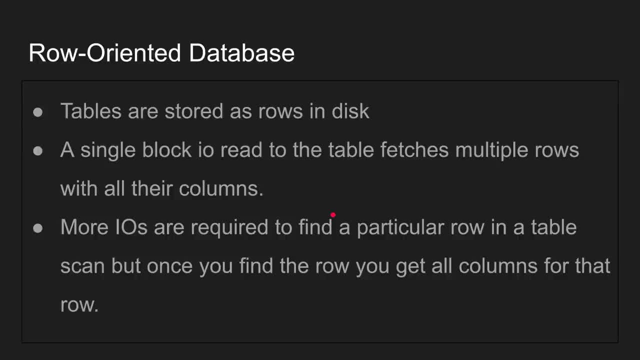 So the first one, row-oriented databases guys. So for row-oriented databases, tables are stored as rows on disk And this might sound a little bit confusing. when you first read it I was like, of course I was saying how else are you going to store stuff in the database You're. 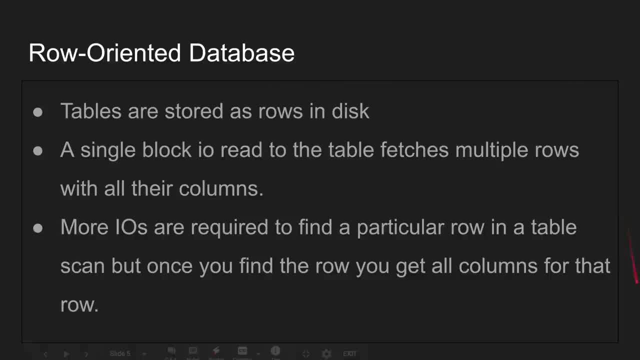 going to store row by row, right? So if you think of the disk as a blob, huge blob, store just things that, just a bunch of bits and bytes, then the rows are just contiguous one after the other: The ID followed by the first name, followed by the second name, followed by the last name. 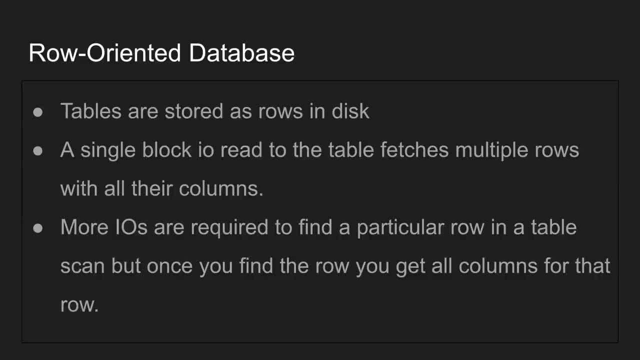 then followed by the social security number, and then comma, and then the second row starts right, And then so on. Each row obviously has a different size. It could be variable size, because I don't know. So, like my name is John Smith and someone else's name Hussein, 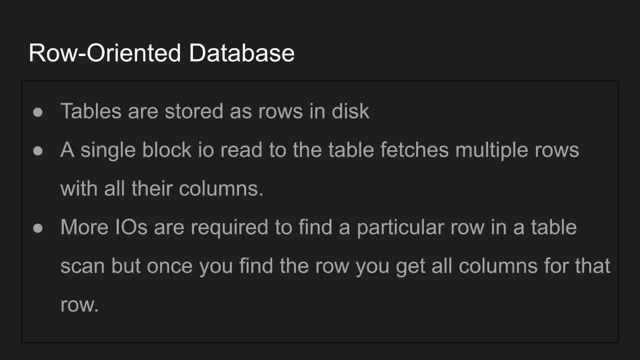 Mohamed Nasser. right, So that's a longer name. So it's going to occupy more storage on disk, obviously, And thus the rows can vary. But for simplicity let's think of it as they're fixed-size rows, all right. 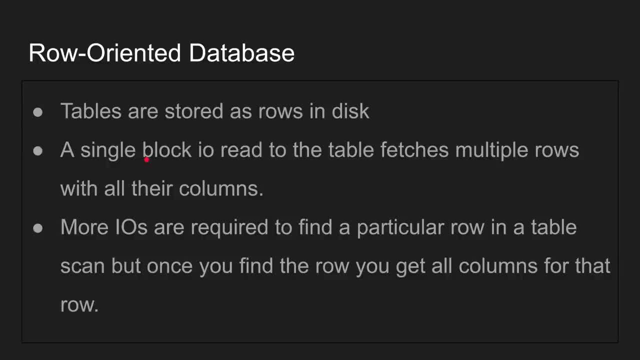 When I want to read a particular row, I go, I do an operation on disk called IO read. When I read that stuff, the controller- whether this is an SSD drive or a hard disk- reads in blocks. It doesn't read like bit by bit. Oh, bit, zero one, zero one. It doesn't read like that, It reads as a block. 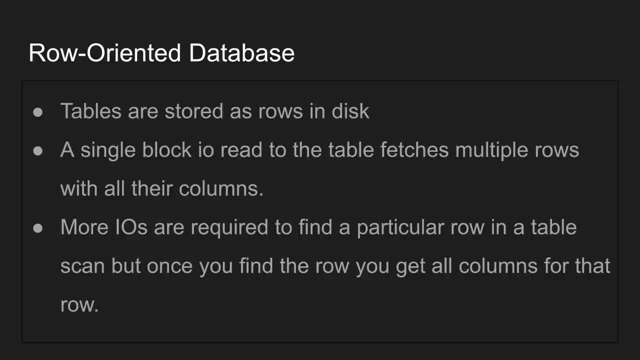 At a time And when you- or I don't know- 1,024 bytes at a time. It depends on the block size. There's something called block size, And once you read that, you're going to get not only one row. 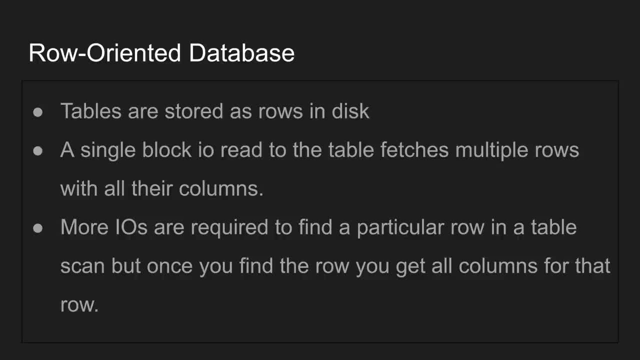 you could get one, two, three, four, five rows in a given block, So you get the act of doing one. IO can give you five rows, And just not all these five rows. five rows and all their columns, all their values. So, whether you want them or not, 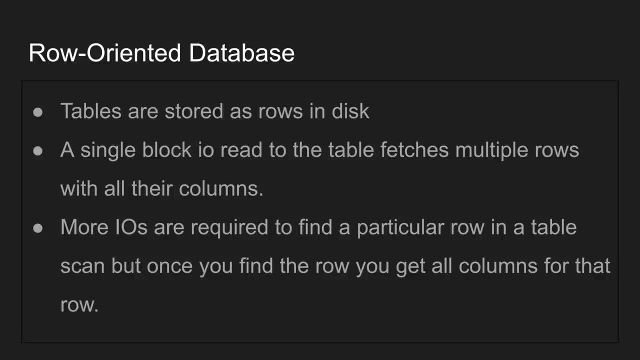 you're going to get everything. You're going to get all the columns, So think about that. So technically you need more IOs to find the row you're looking for. So imagine you're doing a table sequential scan on the entire table. So if you're looking for a employee with social security number 666,. 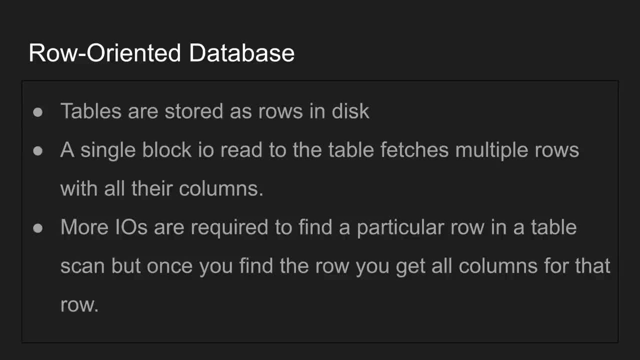 you're going to have to do a block IO. You got I don't know seven rows. then search these rows one by one. You're only interested in the social security, So you're going to only pick that field. Unfortunately, you got all the fields. 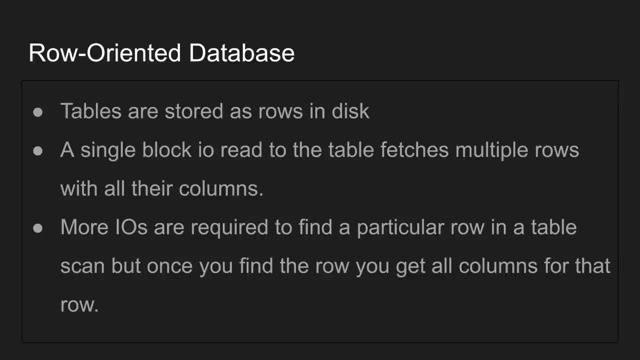 Not saying that's bad. Could be bad, could be good, Depends what you're doing, but that's what you have to work with. So you have to do a lot of IOs to actually get to the row that you're looking for, because you spent a lot of wasteful reads pulling columns that 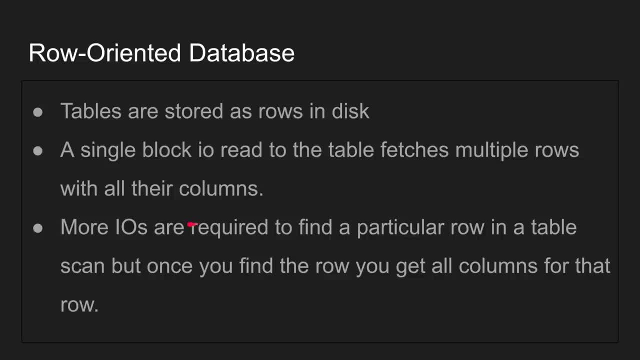 you didn't need and you don't have a choice right. So that's just one thing you have to do. So that's just one thing you have to do. So that's just one thing you have to do. Think about with row oriented. Does that mean they're bad? No, they are beautiful. They are. 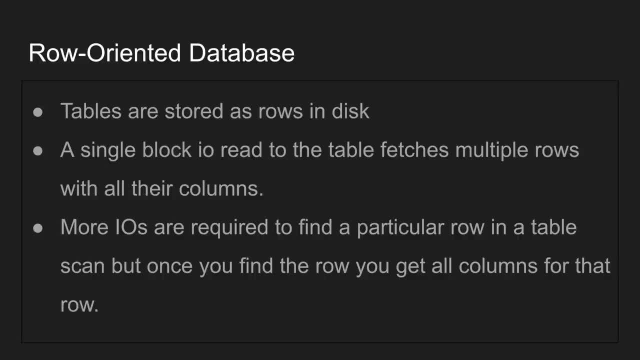 elegantly designed because they are so simple. They are just rows and you can easily think about them. You can easily implement them, compared to what we're going to come up next. So let's dive deep into this. So we're going to take our table and then we're going to convert it into a row. 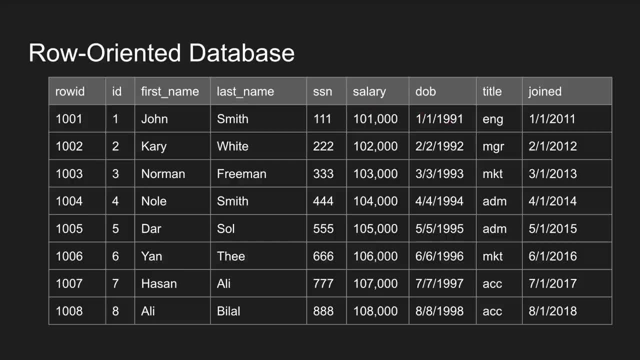 based on desk. How would, how will this look like? Let's take a look. This is how we're going to look like. So imagine this gray box as a block. So we're going to take our table and we're going to 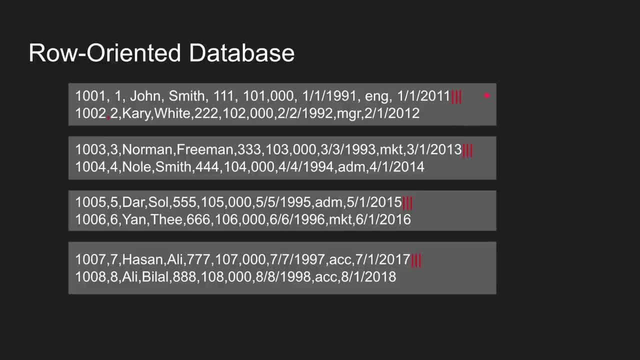 block right And for simplicity I put: I put two rows in the same block. Could be three, could be four, could be five, Who knows? right Depends on the block size. But think about this as as a. 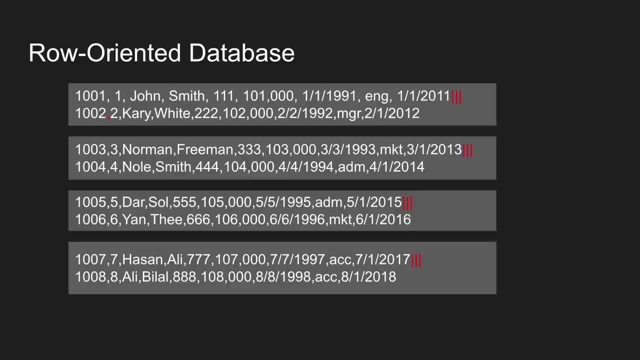 given block. each gray box takes one IO. jump to the controller to pull that block. So once you did you ask for this block. you got everything, son. you got everything right. So now this is how it is stored Basically: the row comma. it's not really comma, it's just literally consequent. 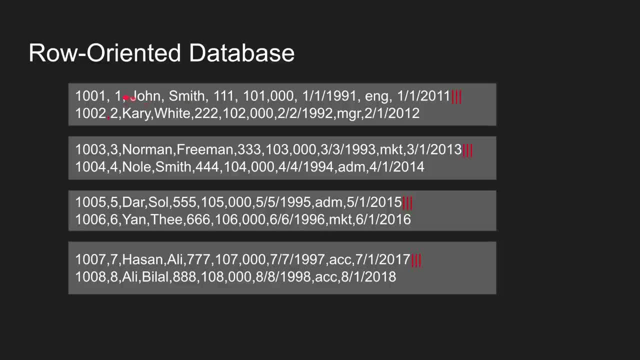 right Values. But I just added comma for you guys to understand that ID, first name, second, last name, SSN, or the salary, birth date, I guess when this John, the occupation and so on, And so you can see that And this. I added this so it can indicate the second row. It doesn't. 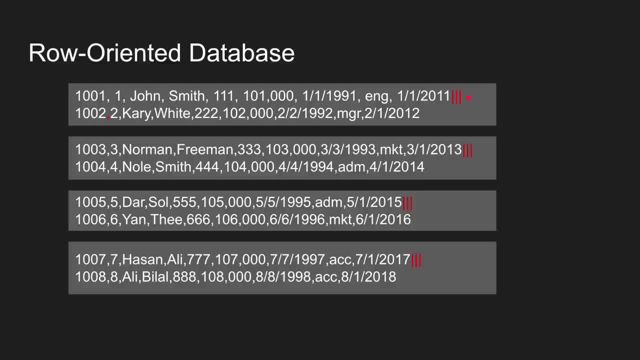 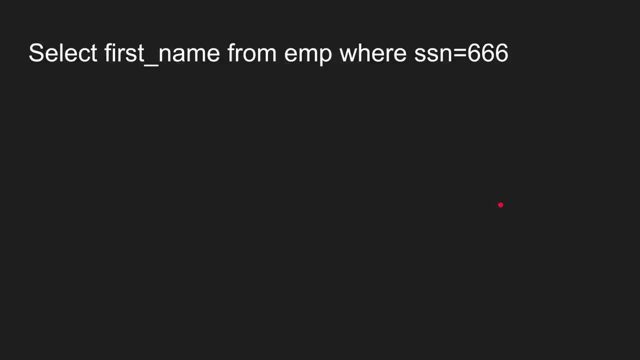 really exist, It's just an identifier like to allow us that. oh, this is actually a second row. Yes, That just started, And then a row just ended, And you can see that we, these are the two rows. two rows, two rows. So let's execute our first query against a 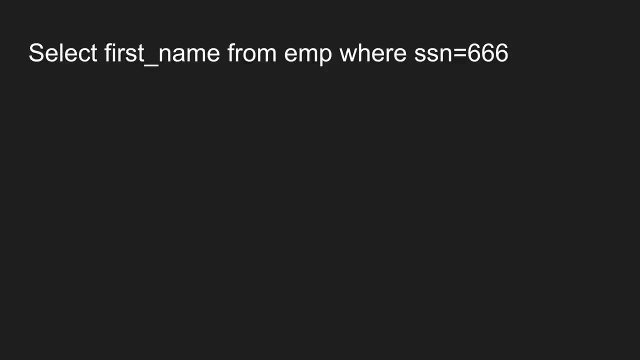 row oriented database. I'm looking for the first name for employee where the their social security number is six, six, six, the devil. All right, So let's pull it. What do we do? We ask: Hey, cause I don't know. I have to start from the top right Because I don't know where. employee. 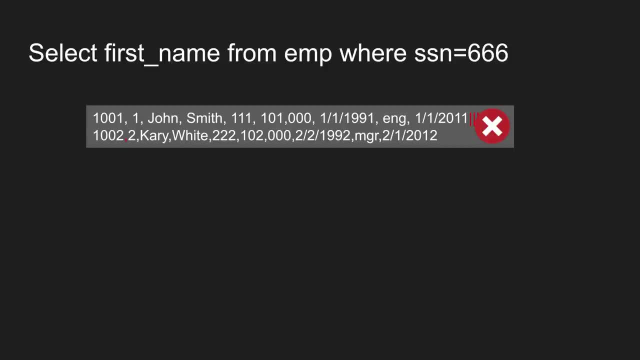 six, six, six is. It's not like that. This number, this field, has any relation to the row itself. It's just a random value, right? So I have to pull the first block of the table. Does six six? 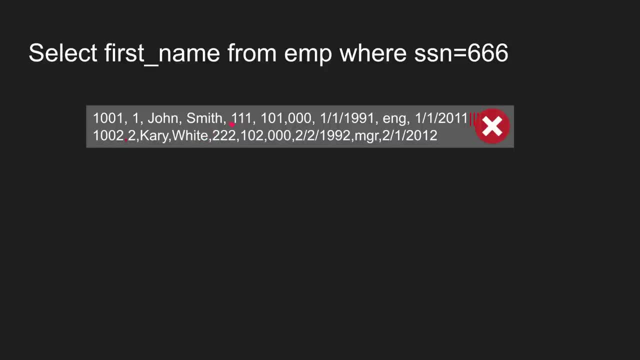 six exist in this. Nope, This is two, two, two And this guy's one, one, one, That's the social security number. So let's pull the second block right. Nope, It doesn't exist. This is four, four, four, three, three, three. Right, And yeah. 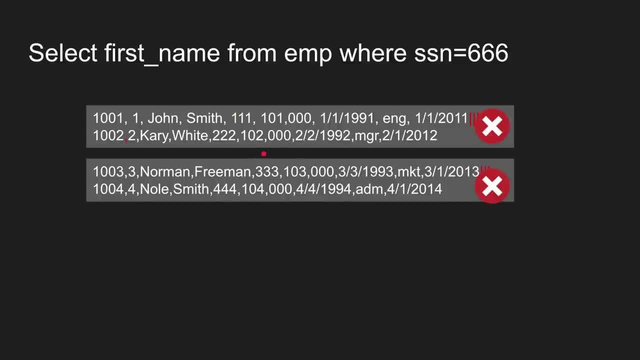 it might look sorted, but it doesn't have to be sorted, guys, Right, Just this is just I'm, I'm, just I'm, I'm walking through that query with you. Right, Again, no, index is nothing. 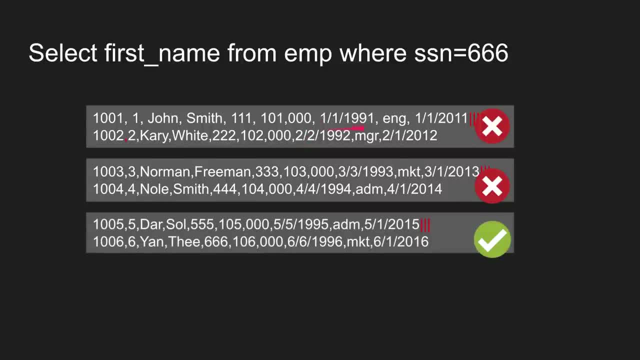 Now I'm going to pull this next block. So I did three reads and then, ah, I happened to find that six, six, six. So I found what I'm looking for Now. I want the first name. Guess what? I don't need to do any extra read. Why? Because the first name is right there. 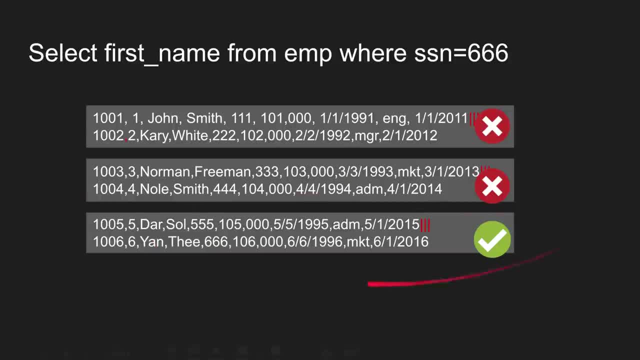 in the memory now, because that once I pull this block, it's in memory, it's in the RAM And when I ask for it I don't have to go back to the desk because, yeah, guess what, I just pulled it. I found it Now. I just- eh, this is the first name And I know because of the position. 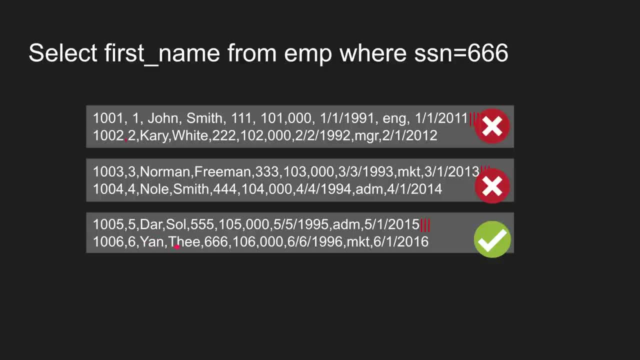 this position. number two is the first name, So pull it So once I find something. asking for extra columns are really cheap, because we we already got them Right. Again, guys, you have to think about this. Whatever I'm going to explain to you, there is no bad or good. There's depends on your use case. 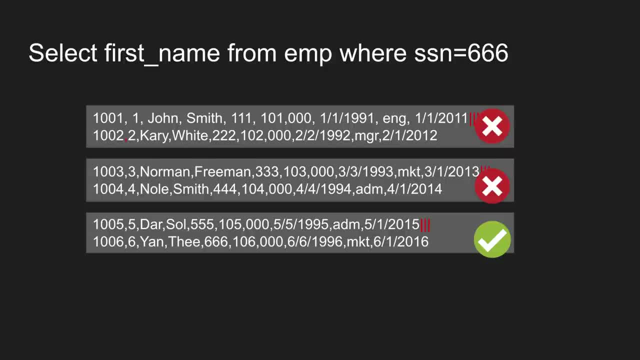 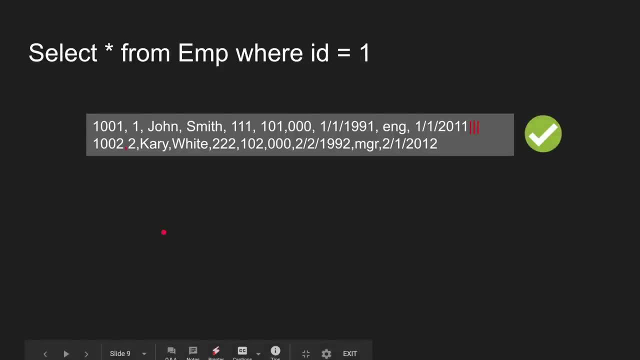 depend on your query, that depends on your where clauses And based on that, you pick row versus column base. We're going to. we're going to come to that. So that's the first query. Let's do another query. Let's do another query. Okay, I guess it's executed immediately, All right, So. 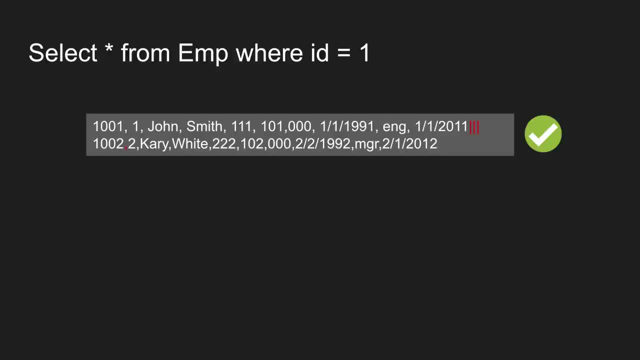 we're going to do select star From employee where ID equal one right. And since it's ID equal one, this, if this is a sequence, the database can do tricks where it can link this sequence with that row. IDS is okay, ID one is on. 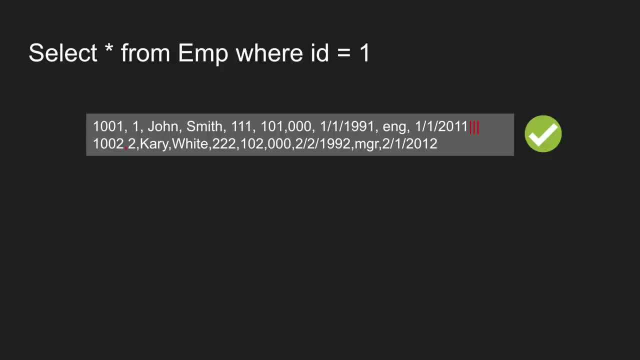 row thousand and one. So I know actually where to jump and pull this row, this block, right. It doesn't have to read other things, but it happened to be that this, the first block, is what we're looking for, So 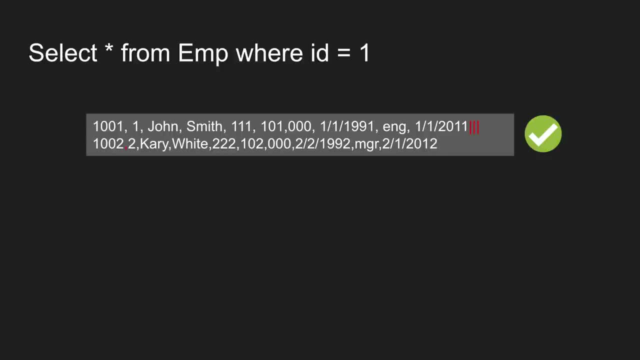 we're lucky, I guess. but even if we don't have this trick where we link the ID to the row ID, we still have to go through each block And once we find the block we want, guess what? Now I want all. 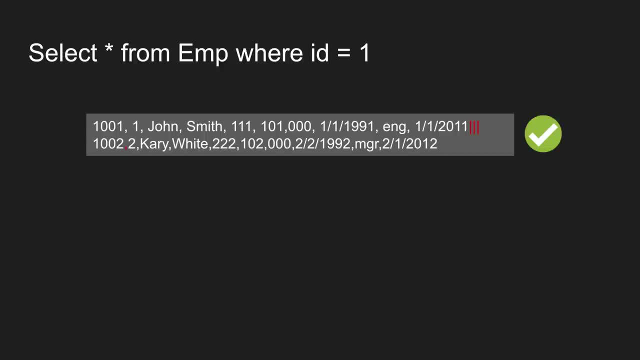 the columns. Can I do this Absolutely. That is so cheap because all the columns are already in memory, Assuming they are not vertically partitioned into another location. right Vertical partition- I talked about that many times in my channels and my courses. So vertical partitioning, where we take 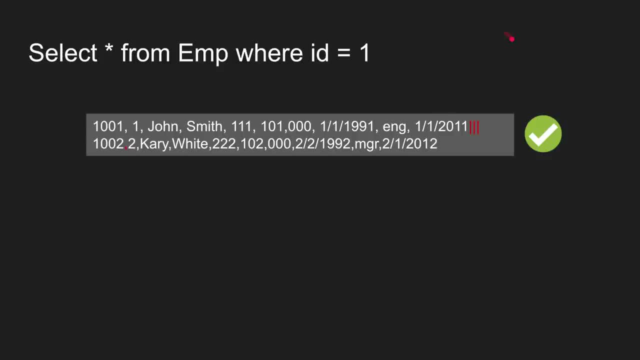 a column and put it somewhere else, right? This is not the case. Well, everything is in one beautiful block. So I pulled that block. I asked for the ID, I found the ID and now the user is asking for every field. I always tell people that, hey, select star is bad guys, stay away from it. But 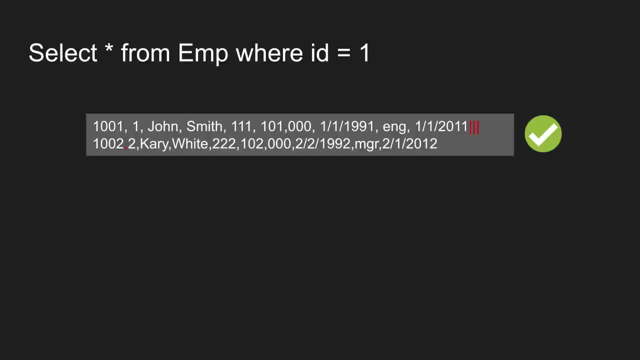 it really depends what you're trying to do. If you have indexes, try to do less of that select star. We're going to learn that it's the worst thing you can do in a column-oriented database. Select star In the row. you can live without it. I guess Still just be aware of that. So that's cheap, That's. 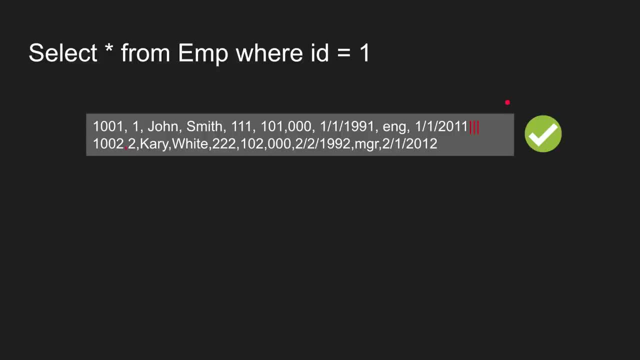 relatively cheap, because I'm going to pull all the rows and everything in memory. Beautiful, Assume it fits in memory. So could it only be one block? Not necessarily because a row can span multiple blocks. if it's too huge, Let's say that we have a I don't know some block. that's too big, Let's say: that we have a. I don't know some block that's too big. Let's say that we have a I don't know. let's say that we have a I don't know some block that's too big. Let's say that we have a I don't know. 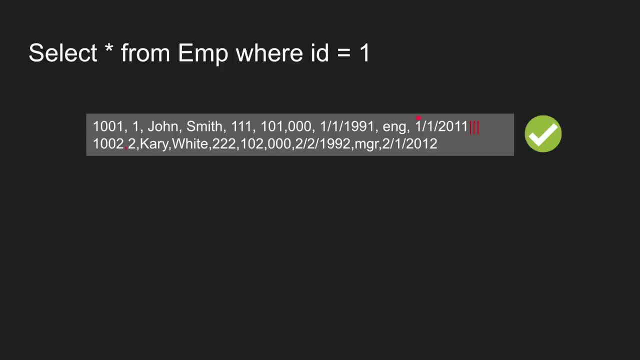 let's say that we have a I don't know some blob here field and then it's a bad idea to store blobs in line anyway. But let's assume you do. But that means this block can, this row can span seven blocks, for example. So you need to read all the block, Not necessarily The database are smart. 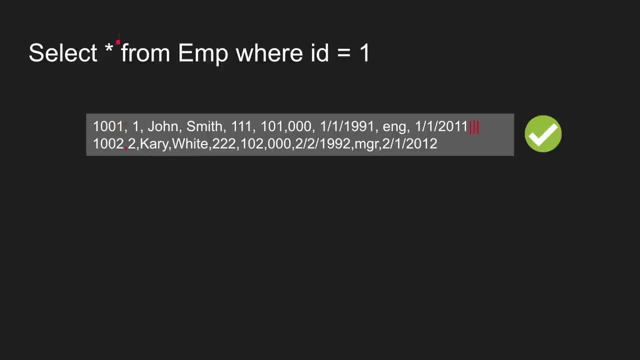 It's going to read the first block, find the ID and only the rows, the columns you asked for is going to ask for the rest of the block to fit your stuff. Databases have been doing this for years. They know what they're doing. But I want to- just I want to explain how I was doing this stuff. 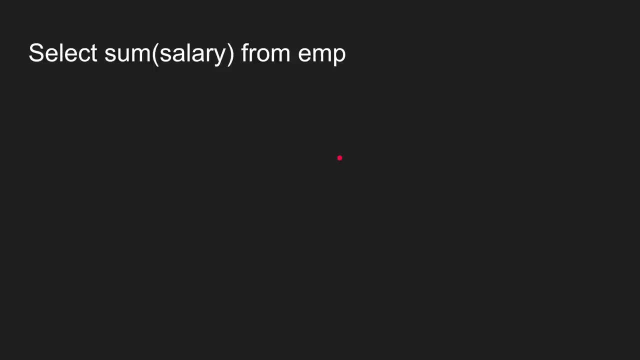 Awesome. So let's do the same thing, but an aggregate. This is called an aggregate function, which is an aggregate, just grouping by something right. So you work on one or few columns, mainly one or less. How do you work with less than a column? That's just an idiot. 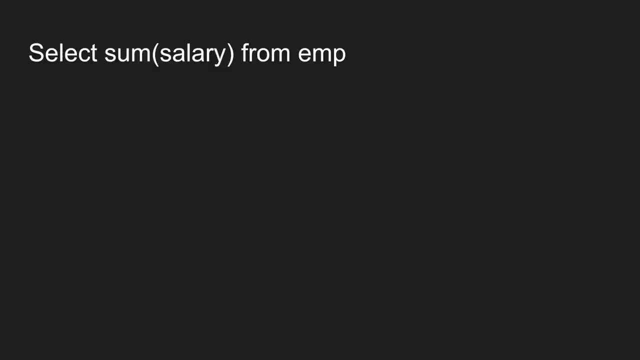 I'm an idiot. Okay, So you work with few columns, all right, Let's say one in this example. okay, So select, sum salary from employees, Just sum every salary. Let's do this So we pick the first block. Well, tough luck. I only wanted a salary, tough luck. 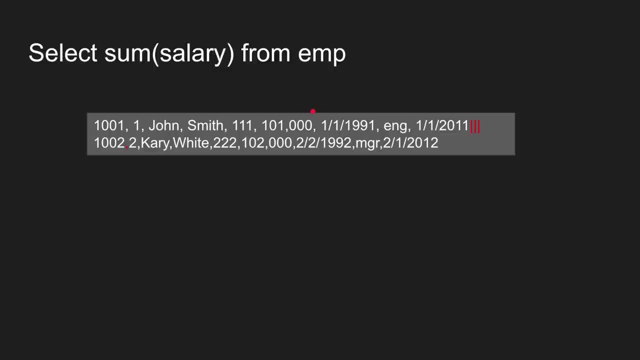 I, I got everything Again, no indexes here. With indexes this could be extremely fast, But I'm I'm just telling you what the database does without indexes. So you pull this. Oh, pick the salary. It's uh, one thousand and one and one thousand and two, So 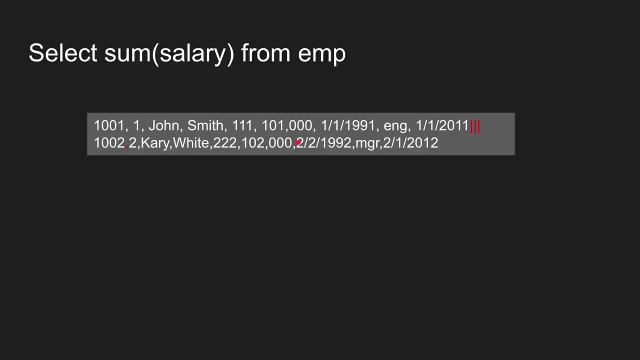 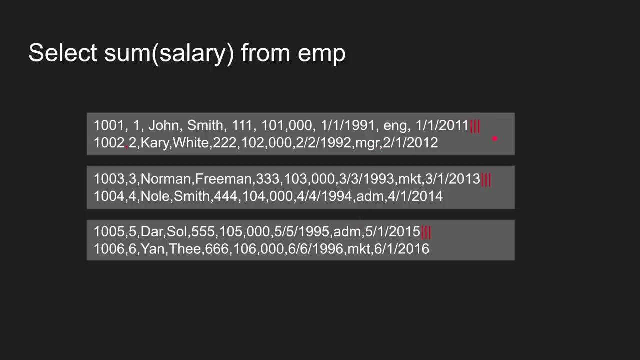 So we summed those two. Now let's pull the next block so we get more rows. Okay, 103, 103K, 104K, sum them. And then pull 105,, 106, sum them. So, guys, every block we pull, we're pulling row IDs, we're pulling first names, we're pulling last names, we're pulling SSN, we're pulling salary, we're pulling that which we never use. 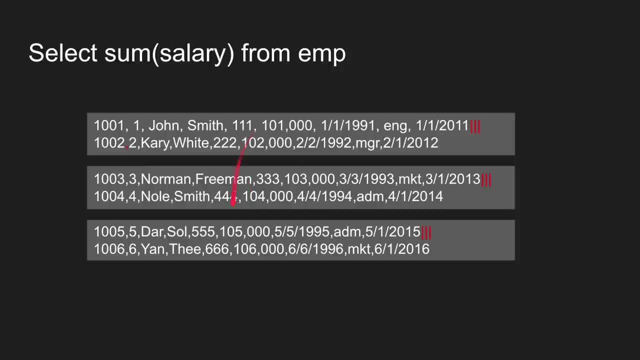 Right. So imagine if I only asked for the salaries and if they were grouped nicely. that would be awesome, wouldn't it? But now, unfortunately, we're asking salary but we're pulling all the rows, So that's a lot of IO. 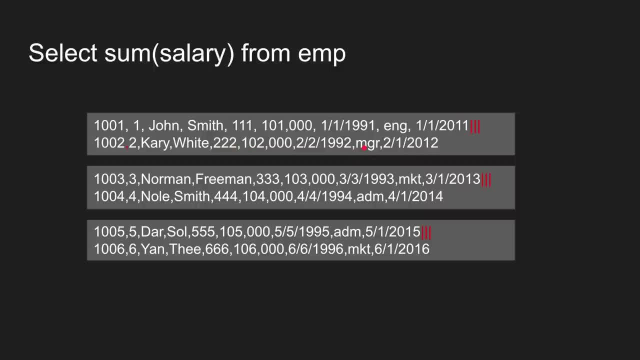 So again, this is not just one read. It can appear in the screen here as a one read If the row is long. you can read seven blocks. So that's seven IOs, right? I mean, yeah, the databases can do tricks where they send one request. 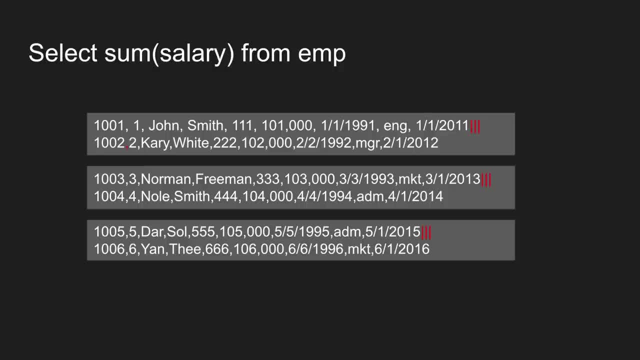 Asynchronously read multiple blocks, But regardless you're hitting the disk, which every time you hit the disk a duck dies, essentially Right. So try to save ducks as much as possible. Save the ducks, guys, Save the ducks. 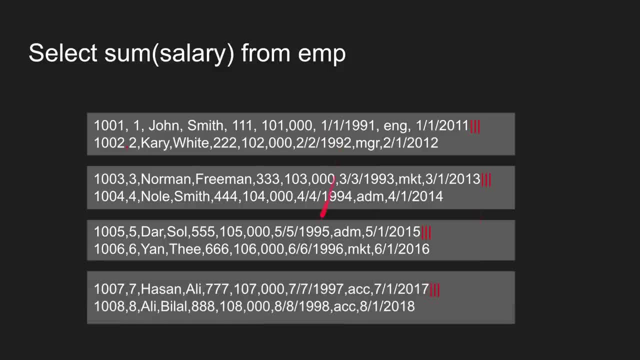 So, yeah, reading, reading And we're summing, We're summing all of that stuff. That's not so bad, I guess. yeah, But you read unnecessary information. That means you almost read the entire table, But you used very, very small portion of it. 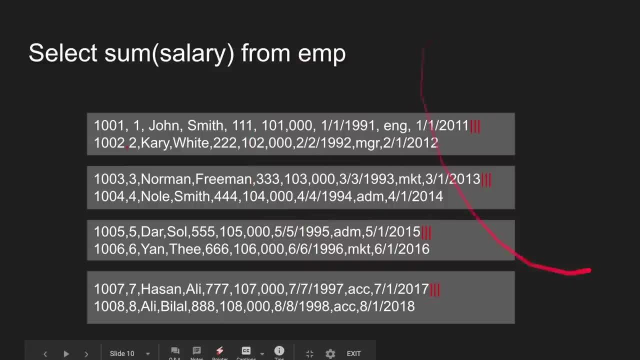 That's extremely inefficient. So row databases doesn't do well this kind of queries. if you think about it, It doesn't mean it's slow. It really depends what you mean by slow. I mean you've run these kind of queries. 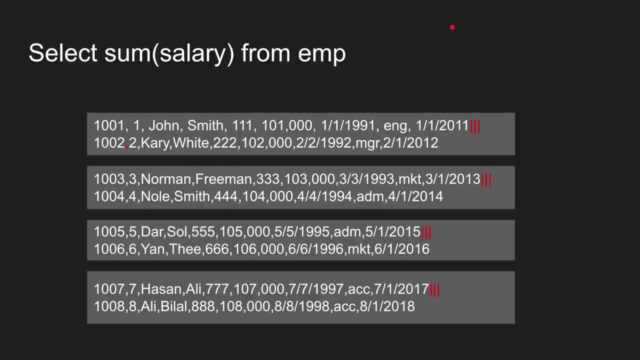 Databases do all kind of tricks to be fast. But if you think about the logic- and I'm not saying This is how databases absolutely work- They have all sorts of tricks. Again, multi-threading: They send multiple threads. Postgres sends multiple threads to read asynchronously. 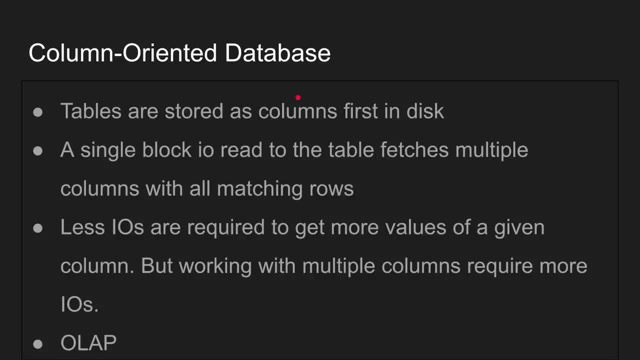 So they do all sorts of tricks to do fast. But let's discuss how column-oriented databases work. So with column-oriented databases, if you think about it, tables are stored as columns first in disk. So think about the first name column, The ID column. 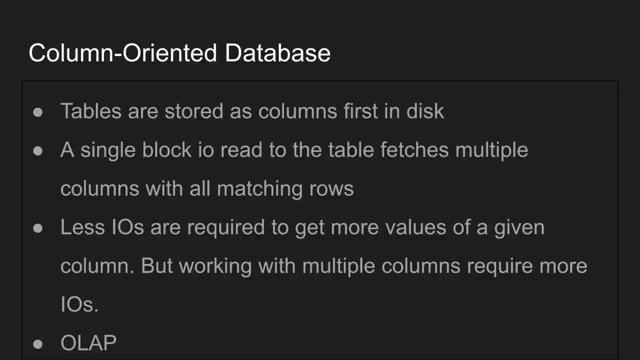 The last name. So what they do is they take the first name and they take all possible values- John, Melissa, Rick, Paul, Hussein, everybody- And pull all of these into and save them in disk as consequent value And then, once that table is done and their last value of the first name is done, they start with the second one. 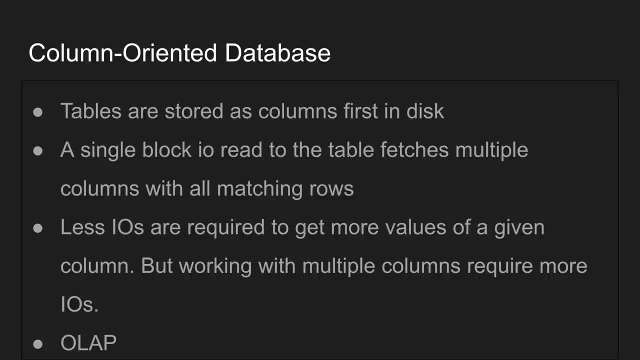 Right, Last name And then so on. So you might say, oh, why are we doing this? And we're going to come to that. So a single block- IO- read to the table- fetches multiple columns with all matching rows Right. 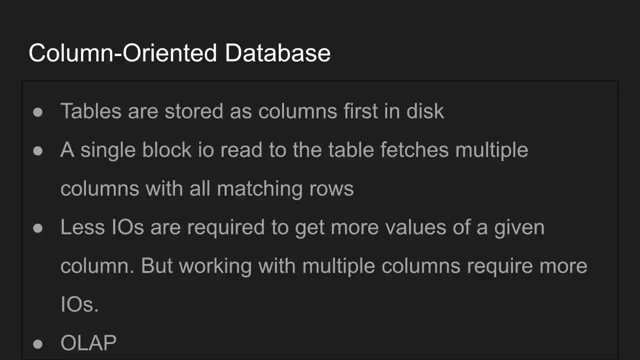 So it fetches a column. It could be fetched one column or multiple, Depends, Right, It depends. Like if you have a small table you can fetch multiple one. If you ask the database to say: hey, give me this. 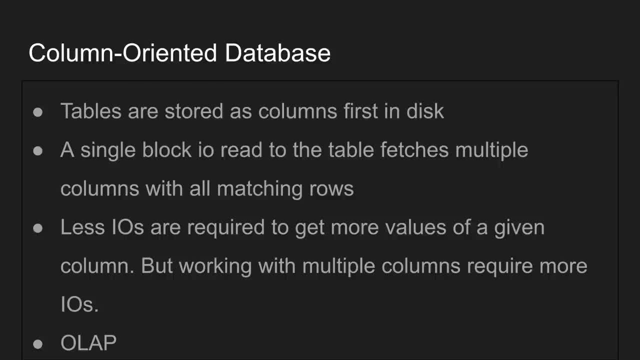 You're going to get a lot of rows. That's the trick here. So a single column with a lot of rows, Less IOs are required to get more values of a given column. Right, Because if you want to get, as we said, the first hundred salaries, that is extremely efficient in column oriented database. 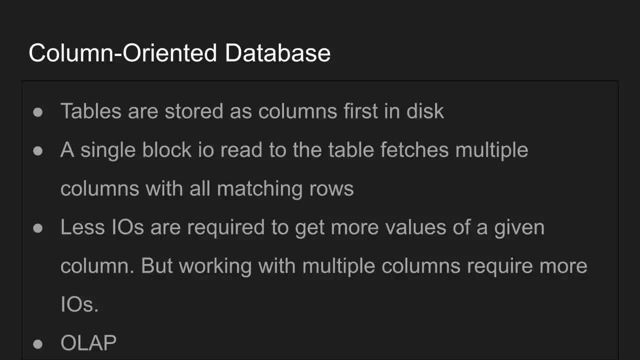 Because, hey, just go to the place where we know we stored the salary column and just walk through there, Because you're going to see the values, Just. consequently, we're going to go to the example- and they are great on online, and I take process, as we're going to see in the coming slides. 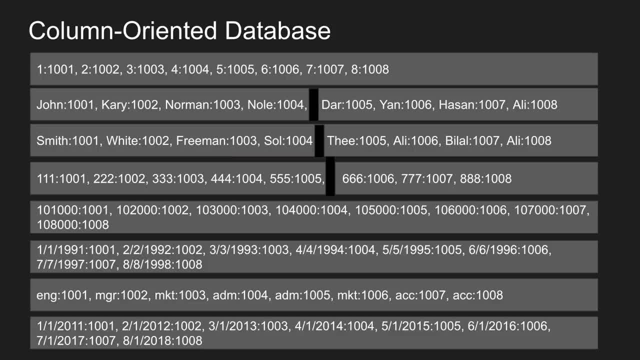 All right. So let's take the same exact table and start as columns. Here's how it looks like. Again, the row ID is very critical here. The ID field is this: This is the first name, Second last name- I keep saying second name- social security number. 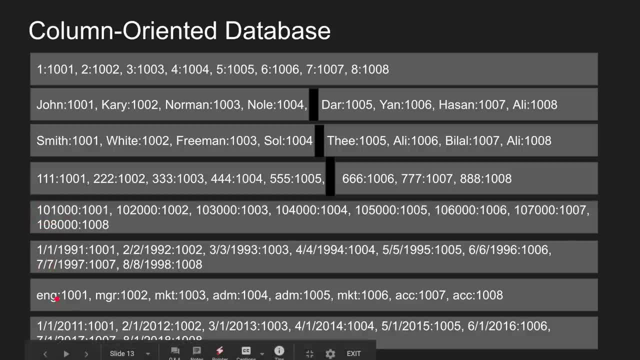 This is a salary, The date of birth, The title, I think, And this is the joint date. Look at this. So Look at this. I want the ID one and this. Which row is this Thousand and one? ID two. 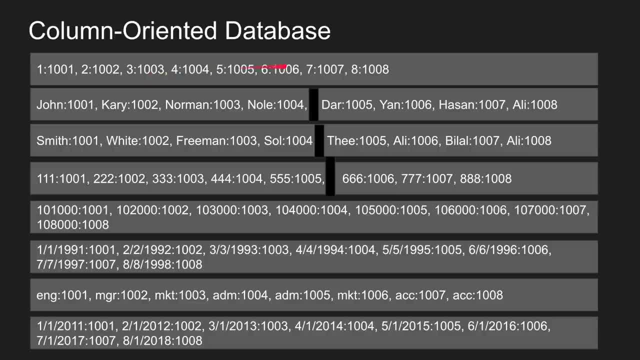 Which row Three, Thousand three, Why We're going to see. Look at this: The row ID is duplicated in every column. So, just like that, What is the first thing that comes to my mind? Oh, editing is going to be painful. 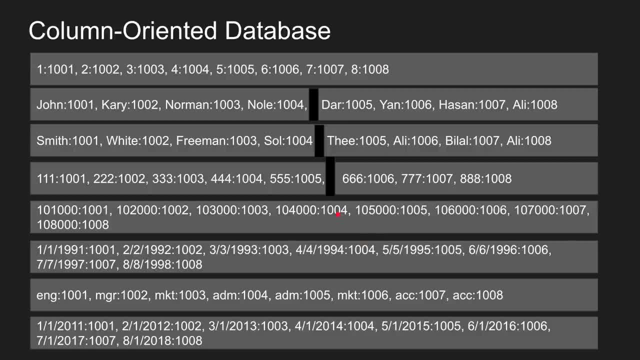 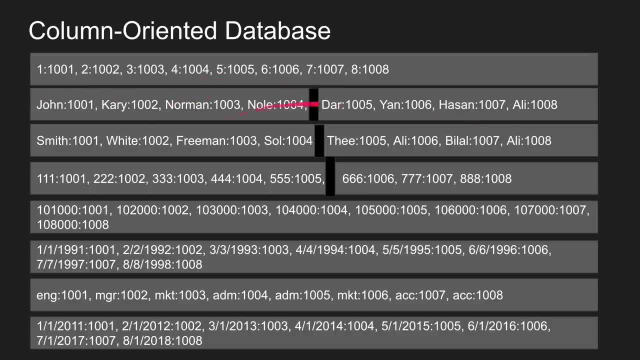 So, and for fun, I split some of them. and multiple blocks doesn't mean they are like. I know this is an integer, for example, or string. I just split them for 10.. You that? Okay, We couldn't store all. 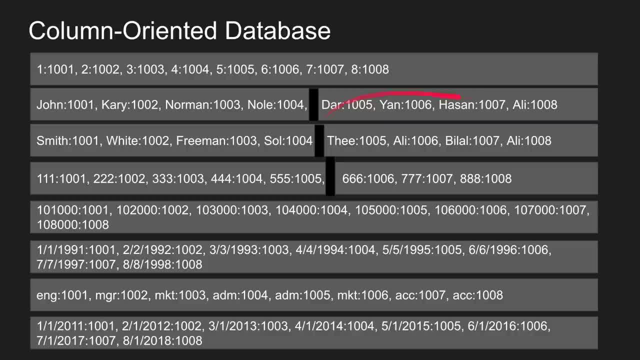 All four rows here in one block, So we had to split it to another block, right? So I can show you different kind of examples. Again, take it with a grain of salt. I've just want to explain this things to you. 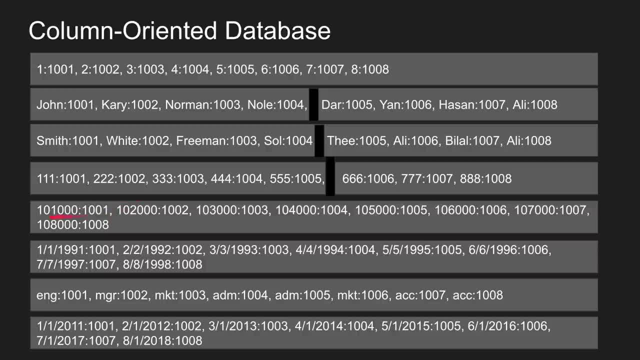 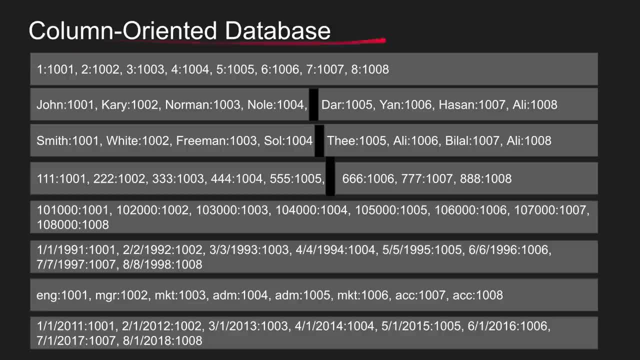 So all the ID fields, the entire, the entire tables here, right All the possible values. So this is not just one block, Could be hundreds of thousands of blocks If you have a lot of rows. Remember everything needs to be updated. 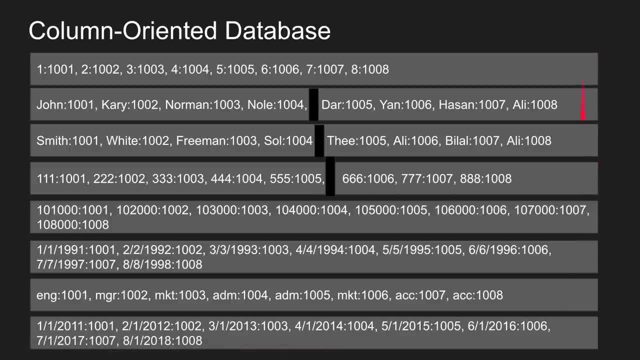 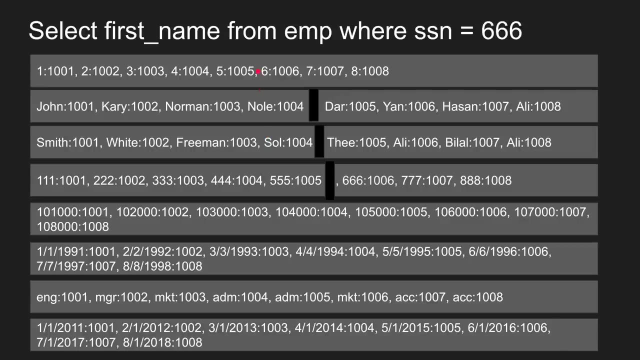 If you add a new row, you have to dead, dead, dead, dead, dead, updated in all of these logical structures. So, what that being said, now we know how this works. let's put it to the test. select first name from employee where social security number 666.. 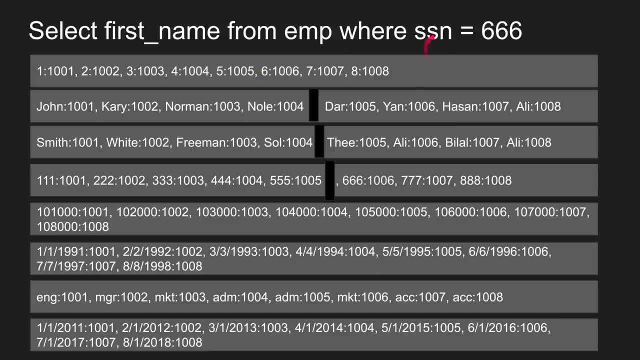 So now the database will say: wait a second, you're looking for social security number. I don't need to look at any of other logical structures Except for the social security which is this puppy. This is the social security data desk, right? 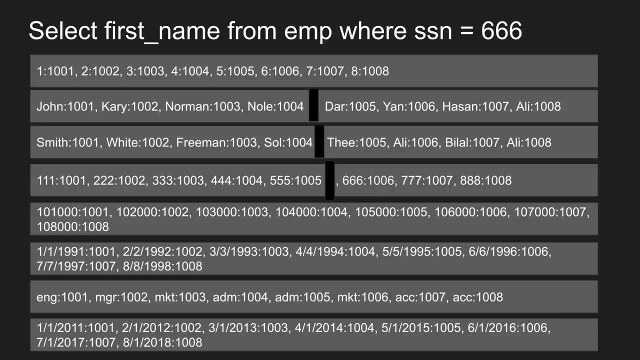 This is how a store. I know this is the location. So in desk I know where to point my needle and read this stuff. So to search for social security number, I only need to pull this right. So now I start reading block by block. 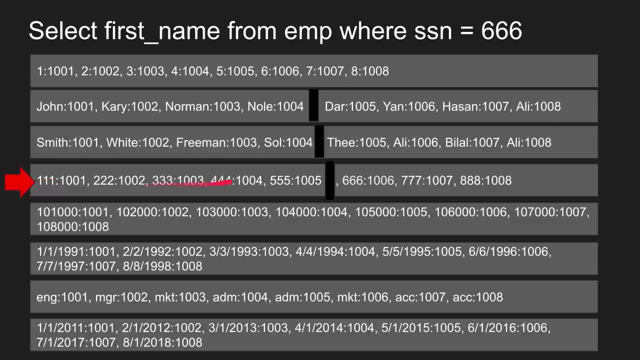 I read first block and I got a lot of beautiful values. I got five, Five, Five, four, four, four, three, three, three, two, two, two, one one. We did not get 666.. So, okay, no problem. 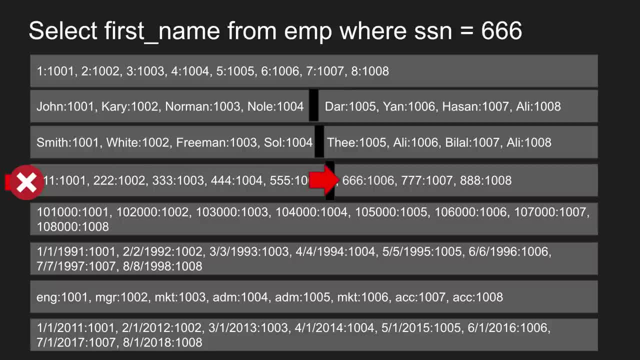 Let's pull the second block. This is almost like the row base, but now at the column level. Does that make sense? So now we got it. We found it, But now I need the first name. What First name is not here, son? 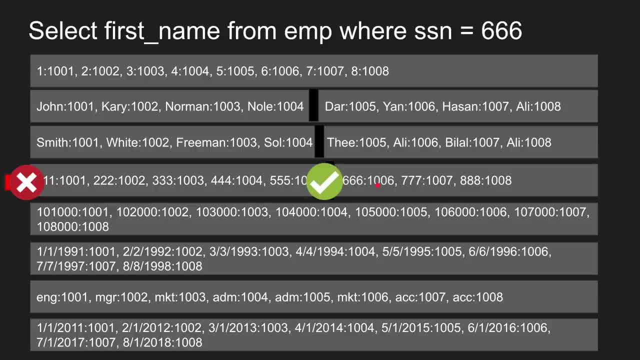 You only got the 666.. Now you found that this is actually 1006.. That's almost like an in how indexing works. If you think about it, this is how Postgres stores indexes. It's actually. if you think about this as an index, it's, it's almost very similar. 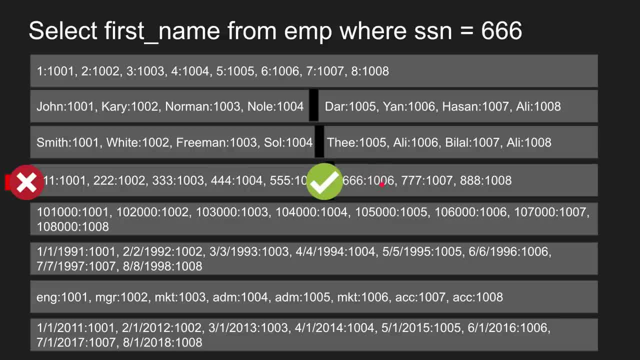 right. It just points to the row Now thousand and six, row thousand six. I know this value, I know the role I'm looking for. This is very critical and I'm asked for the first name. Where's the first name? 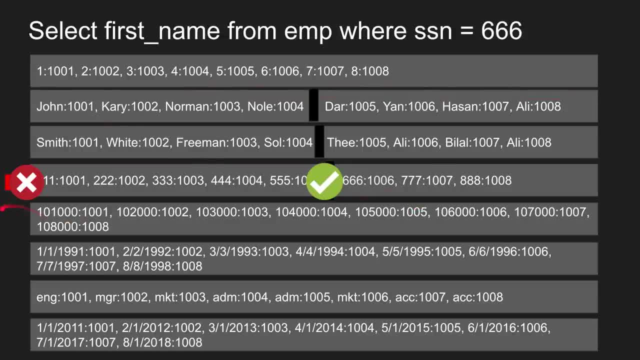 The first name is right here. This is the first name, So I'm not going. I'm going to read these law, I'm only going to jump right here, right. So obviously we found this row as we said, and then we can jump right. 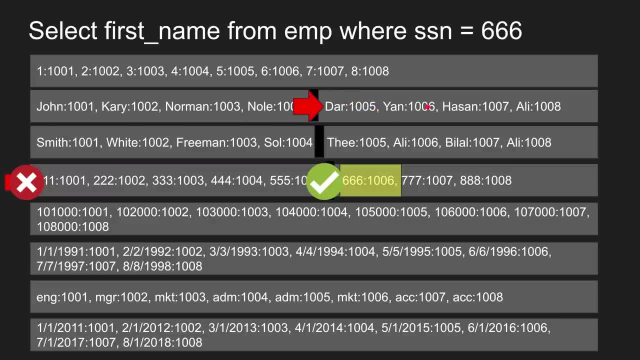 Not the first block. I'm going to jump to this block. You might say, Hussein, how did you know that it's in this block And you didn't pull this block? because I know the row number and the database does all sorts of trick to to. so, okay, this block has only rose from 1,001 to the 1,004, right. 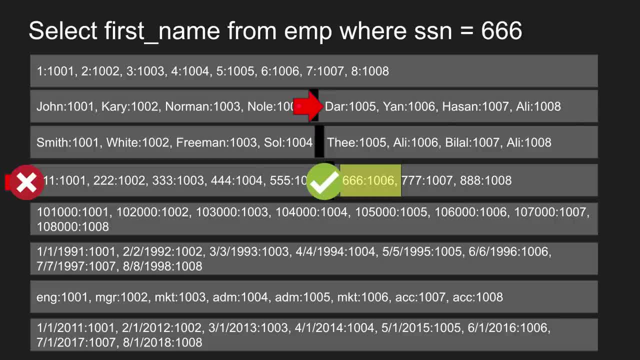 So I'm going to jump to block number 703 because it exactly locate the row I want. right, Because they have all this metadata mumbo jumbo, right Again. that's back to the our question. the 1,006 link with a block is all there. 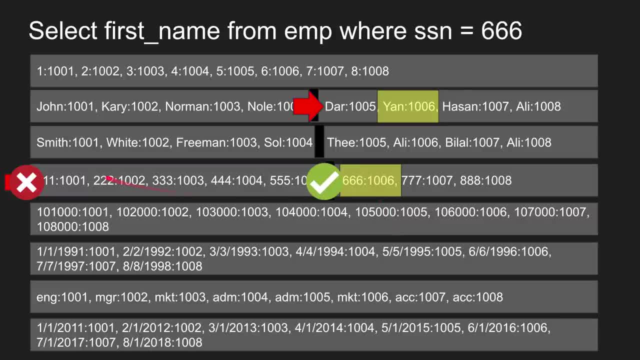 They know they pull it and they find it. So we had to do one jump, one block read, second block read, jumped back to another block read, and then we got it. So three. Yeah, that's so bad. 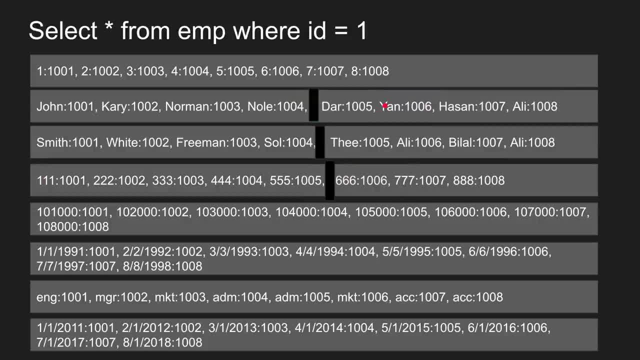 I guess let's just like store from employee where ID equal And let's see how, how, how calm, how, our beautiful column, index, column, storage do All right. So ID equal, one again. I don't have any knowledge with this. 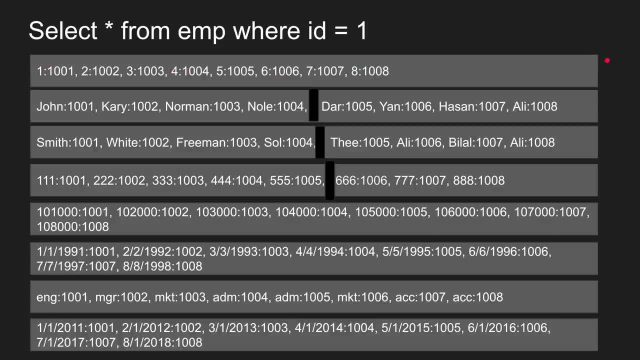 So I'm going to start ID Where's ID? This is the ID, So I need only to read these structures right, Let's pull. it found 1,001, it's 1,001.. So now I have knowledge of the role. 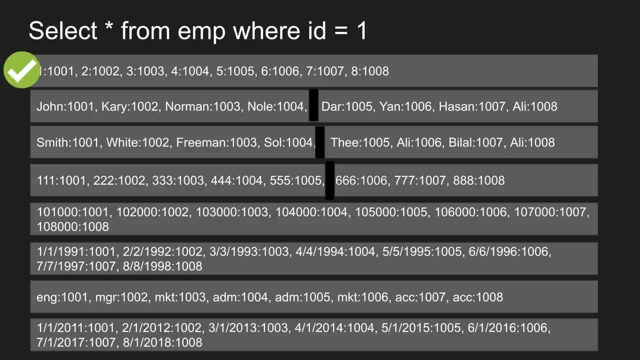 I know which block to read, but the user asked me for everything. Okay, Let's jump on. Okay, We found that Let's jump onto the first name. We know which block to read, So this one, that's one, read, let's jump on. 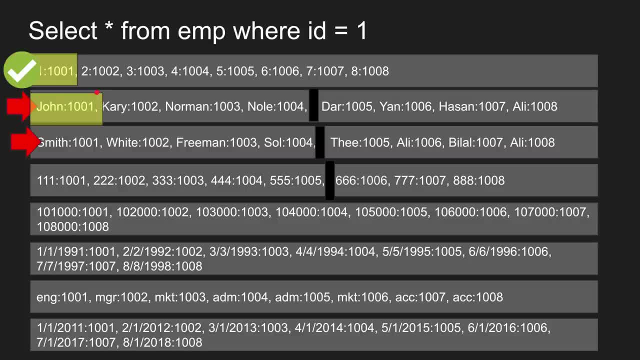 No other IO last name, because they want the last name, They want everything Read. Oh, found it, Because I know I don't need to read this, because I only know which block exactly in each column to breed to find my value. 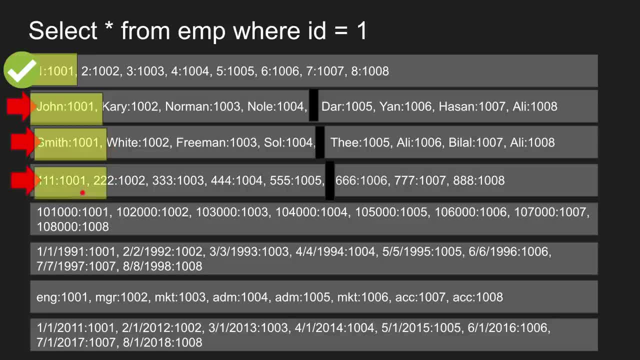 All right, SSN: find read salary read birthday read engineer. Oh, I have a bug here. I should have- I didn't stretch it enough- engineer read and joined it Read. What have we done, guys? This is the worst query. 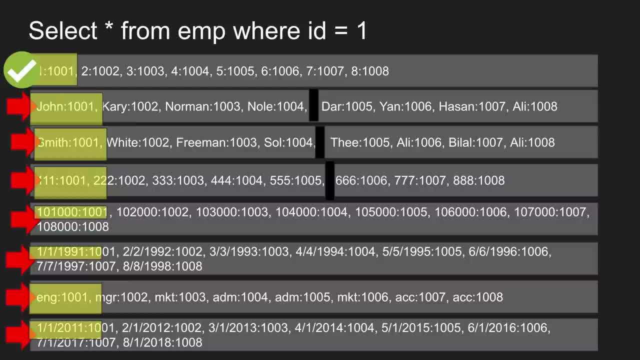 There is so much thrashing happening on disc that this is the worst thing you can do. Column databases just tanks when you do this, especially if you have a lot of columns and you're asking for everything And if, if, especially if you have like a lot of uh and queries or or queries. 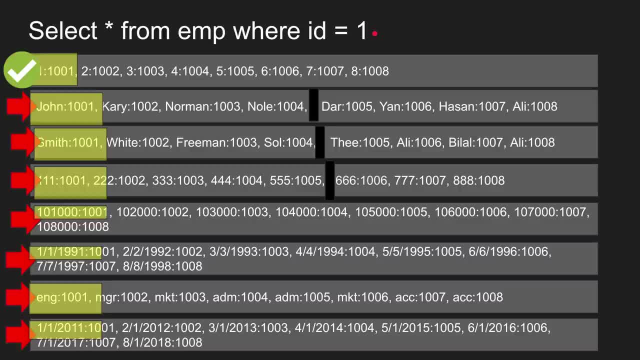 here where you had to jump to find the multiple rows. Ooh, That will, dude, dude, do that, dude And do that. I'm talking to both of you, dude, do that. Do not do this. select star with a row storage. column storage. 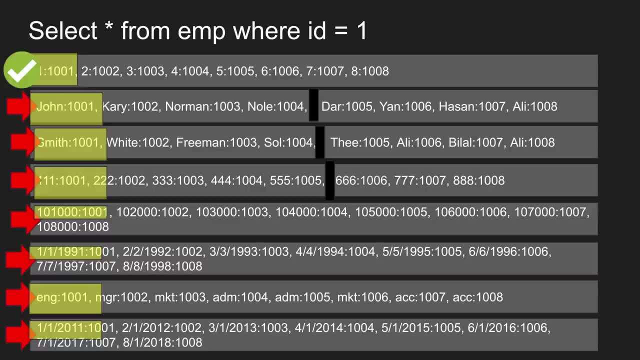 Do not do select star. This is: do you know how how many ducks die? When you do this kind of queries, guys? you go to the database. you read all these things: ducks- every IO kills a duck, right? 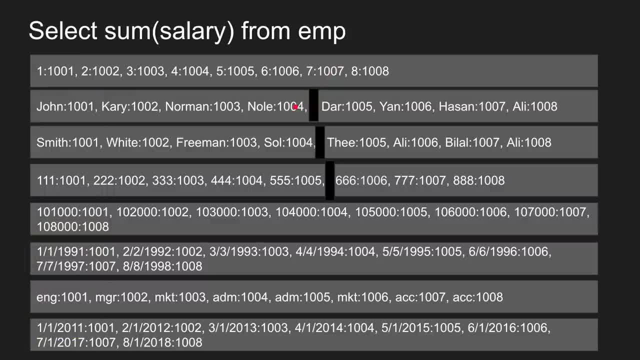 Save the ducks please, Guys. All right, Let's Do this: select some salary from employees. Now that we saw how horrible column oriented databases can be, Let's see how great they are. I want to sum all the salaries. Yes, sir. 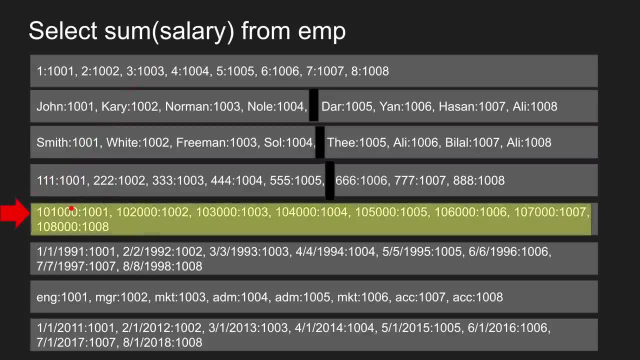 Where's the salary field There? it is One read, done, done. Well, if you have, if you live in multiple blocks, you're going to read the multiple blocks, but done, That's it. That's it. And if you have caching and stuff like that- and by the way, I didn't mention 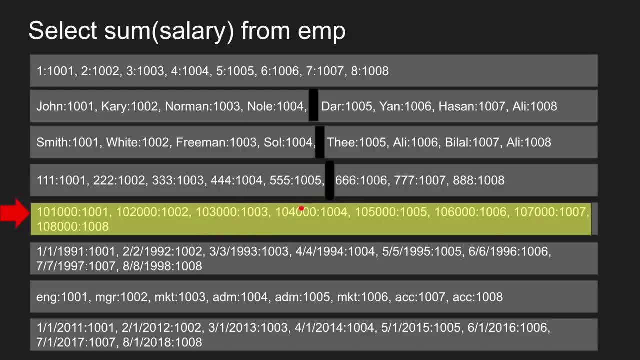 something. If you, if people, multiple people, have the same salary, column, oriented databases do something called compression and aggregate They actually if, let's say, if, if, uh, if three people have a hundred thousand salary calories, okay, All of them have a lot of calories, right? 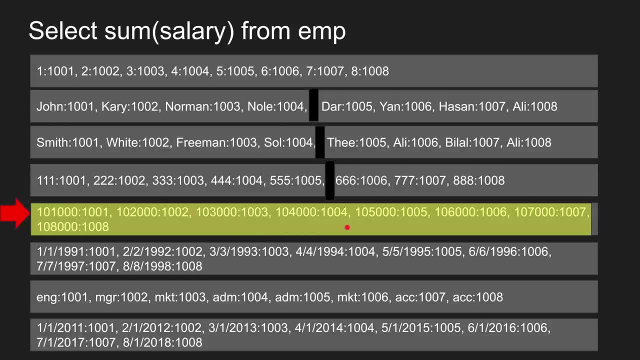 So I have a lot of salaries and then you can- you can Just have one entry- 100,000- with a comma base. I said 1,003,, 1,004,, 1,005, all of them have the same one. 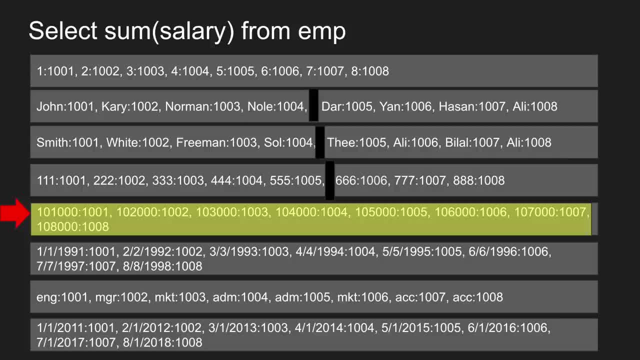 So this is even more compact. So this will give me a lot of bang for my buck by just doing one block Again. I sometimes if, I, if, if, if there's like a duplication, Ooh, this is the best thing for common. 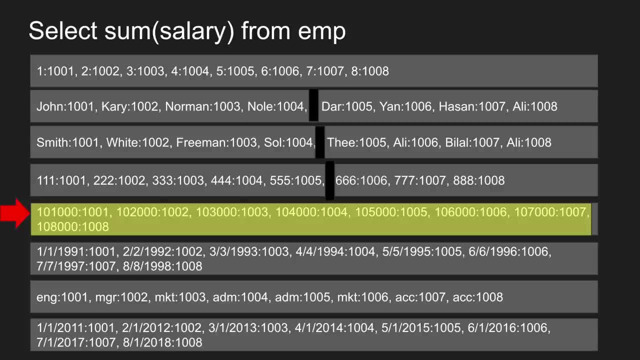 oriented database that you just shove it in the same row because they're okay. They were going to do it as an array. We talked about that a little bit in in my post-class- 13 post-class. They just started doing this, uh, index de-duplication. I believe they called it B3 D. 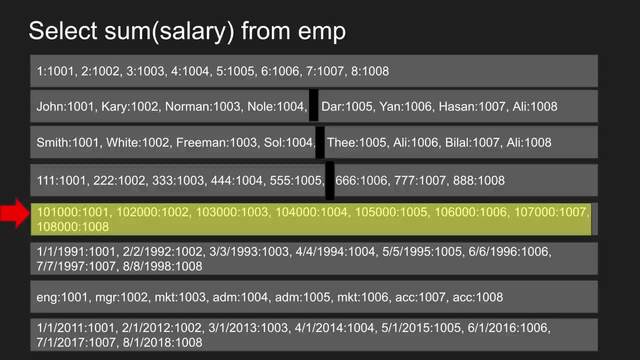 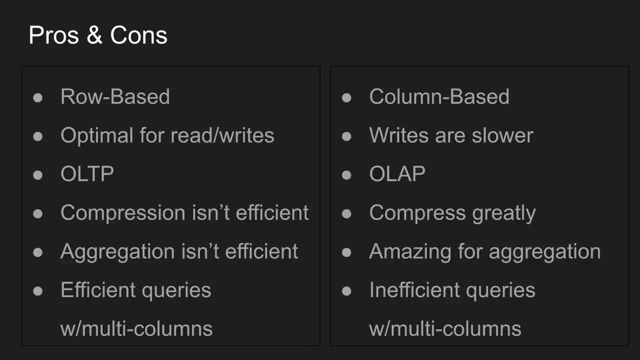 duplication, Postgres, the version 13, they start shoving more duplicated values in a single leaf node so they can compress, compress on. So yeah, pros and cons, Is this thing perfect? Nope, nope, nope, nope. 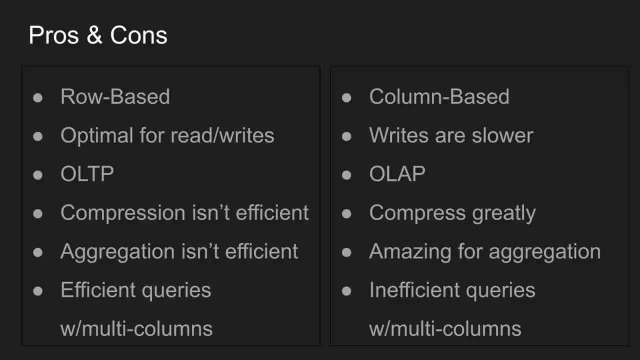 Nothing perfect. It depends on your use case, guys. Uh, if you ask me, I still Prefer row based. to be honest, just simplicity of writes and reads, but there are some cases where you need column based, oriented to summarize right. 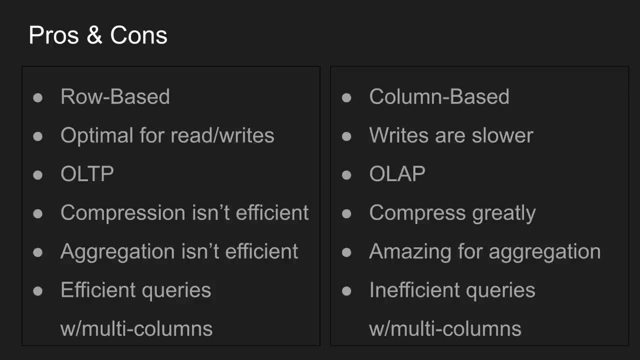 Right And reads. you want a simple structure and we saw how complex column stores are right, They're very complex, They. we have to duplicate the. you have to show the, the, the, the, the, the row IDs everywhere. 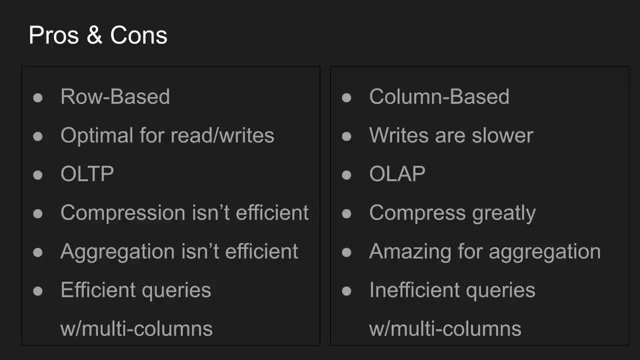 That can be a little bit messy for rights And slow writes and reads right. That's why a lot of people use column based and and warehouses and stuff like that And lakes, data lakes, where things are just almost static, They don't edit. 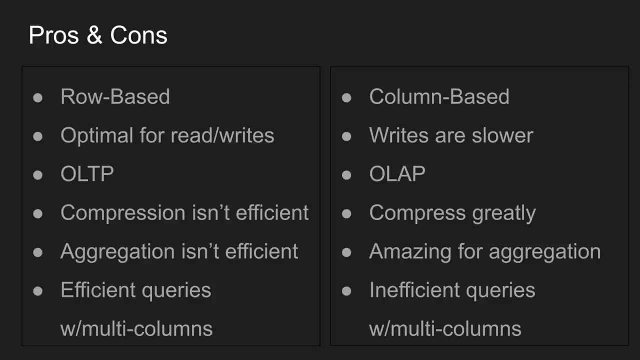 They just do a lot of analytics on a single column. So that's powerful stuff, right. So let's go through these pros and cons in general. So for row based, uh, it's very optimal for read and writes, right? And then, uh, well, I'm going to say read and write, I'm going to say transactions in general on online transactional. 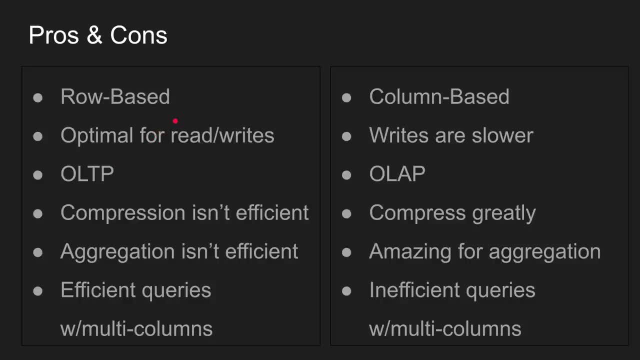 processing right. They are very great for this because, uh, they are very simple in their implementation. So, and if something's simple, we can enhance it and make it more and more efficient as as we go right. That's why your rights are fast. 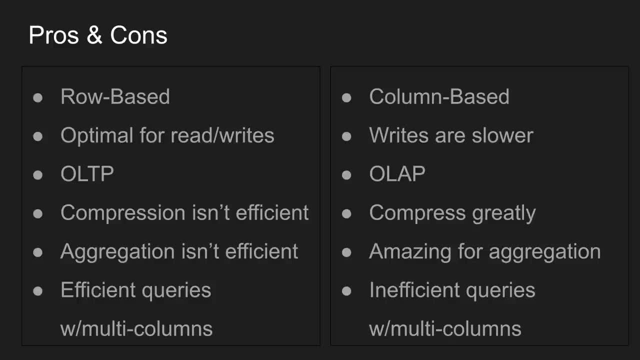 They were uh reads almost fast. It depends what you, how your query looks like. We saw some examples: right Online trends, trends. uh, online transaction protocols and processing. right Transactions are great for row based because you start a transaction. 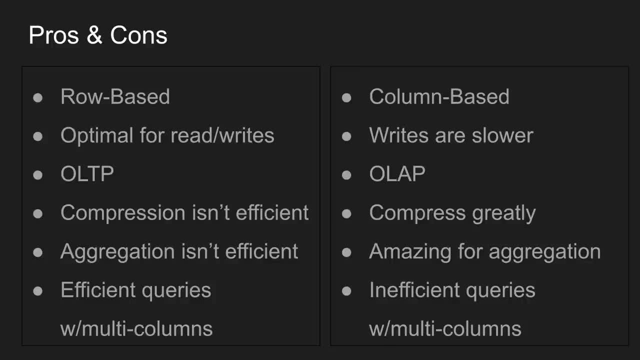 We know what, exactly, what rows, what blocks to touch. We can uh write the wall, uh the the right ahead log efficiently because we know exactly what we're changing right Versus column. This will a little bit. the structure is all over the place. 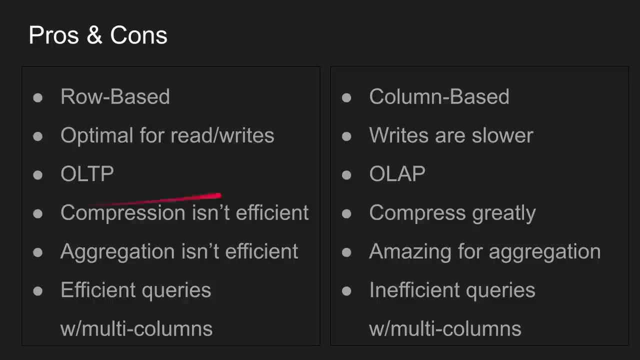 So we have to do a scatter shot. Compression isn't really as effective though, because- uh, think about it right. I'm not talking about the the do duplication. That's something you can do in the index. I'm talking about 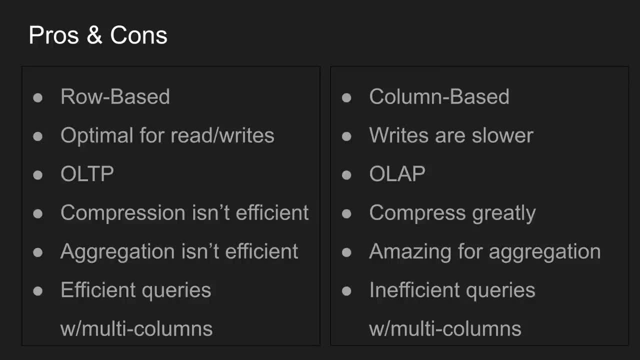 Just the idea of having the values, uh, in the in the row. the row itself is almost distinct, right? It's almost like a hash, because they it consists of different fields, right? So you can't really easily compress it, right? 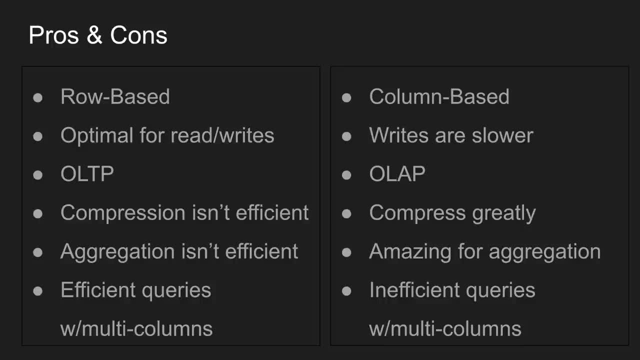 The compression algorithms is not going to find a lot of tweaks to compress because the values are are not Consequence right. Compared to uh, the column oriented where the are they, the consequent values, are almost the same type and almost the same thing, right. 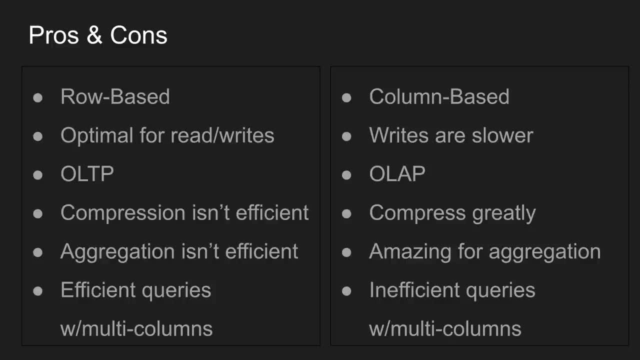 So you're going to get a lot of chances where of duplication, like, you get a little a lot of people named John, right? So John's are going to be swash squashed together. So compression is not as efficient with roles because you you get all this different things that are 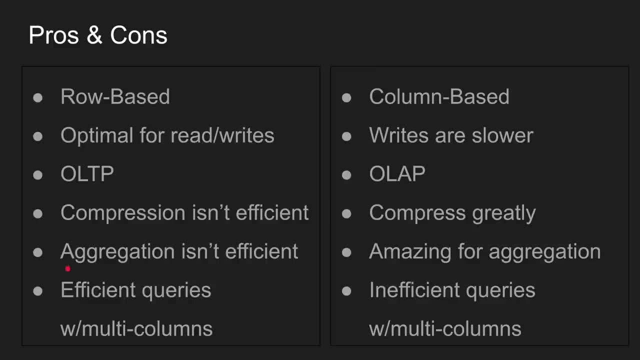 Next to each other. Right, I know completely different. So we can't compress as effectively aggregation. We saw how, how, how poorly the role based database did with uh, with the aggregation. I mean we had to query the whole table, but we we pulled lots of information that we didn't pick. 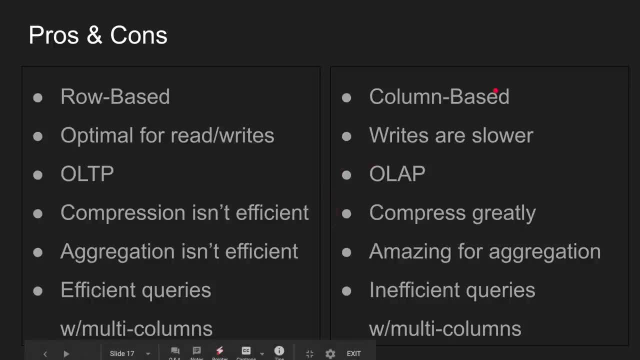 So column oriented databases were more efficient when it comes to with aggregation, because we fetch only what we need and we we work on that. So if you, if you started switching Information or data that that are only what you need, then you're going to start you, you'd be very, very efficient in your query and you only fetch the information that you need. 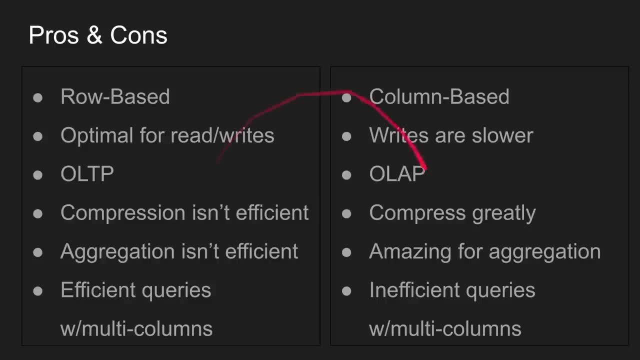 Right. So obviously you're going to have a lot and you're going to finish faster than than raw or oriented databases. efficient inquiries with multi columns- right? So if you're picking multiple columns in a query or working with multiple columns usually, 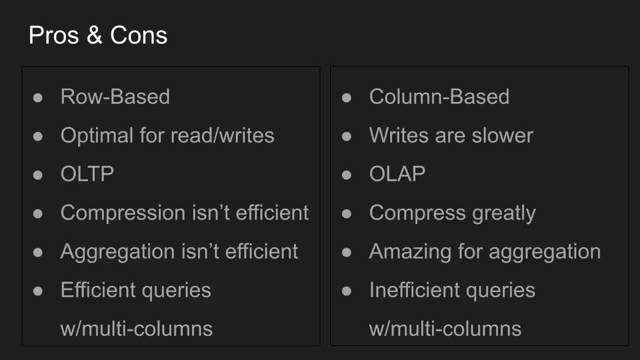 If you're picking multiple columns in a query or working with multiple columns- usually Row oriented or better Right, And again it depends on talking only about the query itself, right? So you can have a lot of columns if you want to, but if you're only working with a few of them, that's absolutely fine with column oriented databases. 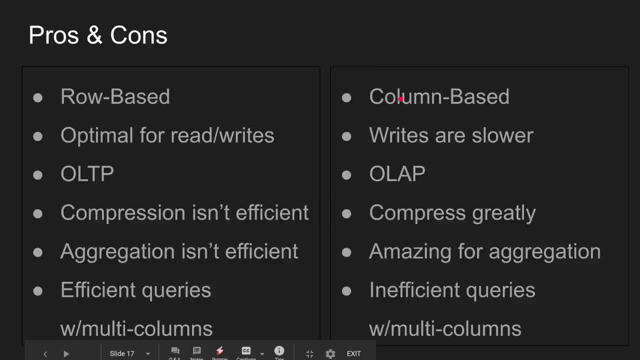 But if you're actually working and touching all these columns, that can be bad. Right With the column oriented database, with with raw, we saw it Right. a fetch on the row give us almost all the columns against. again, you, if you, unless you have vertical, 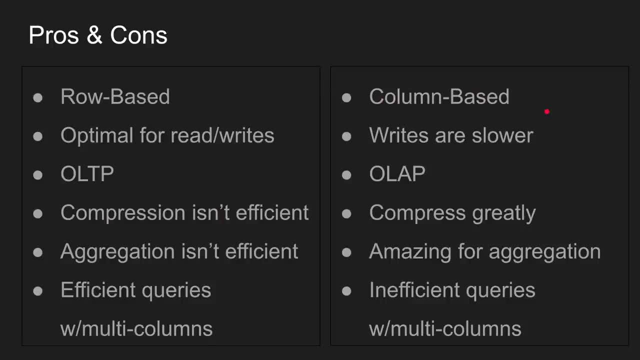 partitioning. so with column based, writes are slower because we have to update all these beautiful structures. every column has almost a structure on itself. think of it this way. how is it stored? so i need to know where is it located and touch it, touch it. touch it every column right like very 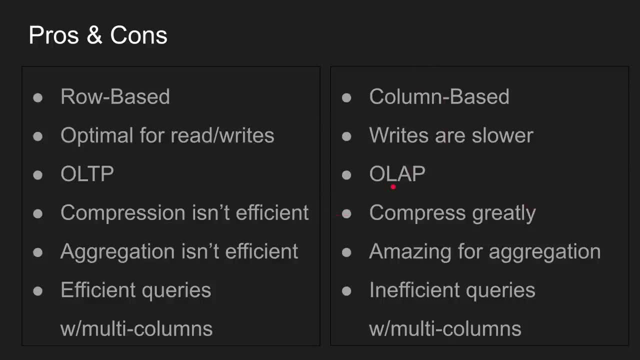 similar to indexes. if you think about they are perfect for online analytical processing. so if you're doing analysis, you're not touching, you're not writing perfect column around the database. it compresses greatly because all similar sampling are together so you can the. the compression algorithms can do magic on these things and compress them. amazing for aggregation. we saw 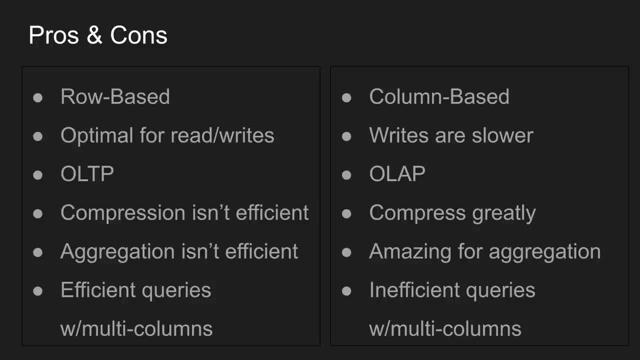 done. right, that was that was. that was amazing. i'm gonna, i'm gonna, i'm gonna admit. and finally, it's inefficient for queries with multiple comments. if you're working, if you're asking for a lot of columns, don't do a column, don't do column oriented. i know this is a little bit weird. 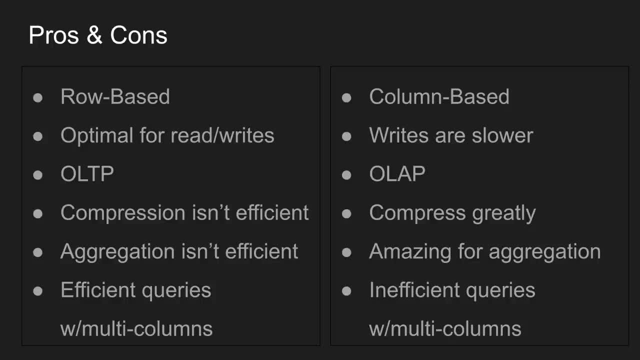 you think that column oriented databases or column oriented data stores or columnar will be great if you're asking for a lot of columns? nope, they are the worst of this stuff. i know guys, uh, postgres, mysql, other databases- most of them are row based storage, however, sap, hana and 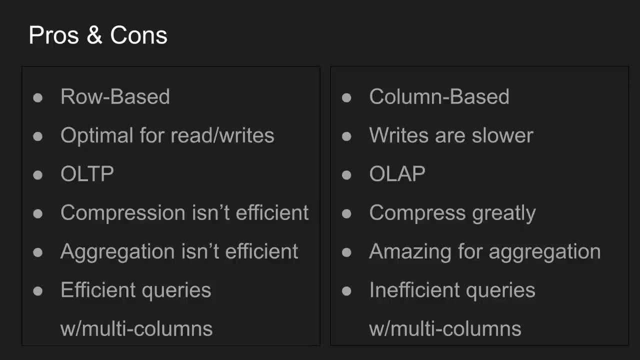 others have. uh, oracle, i believe most databases by default go with road row row based storage. however, if you think about it, they have database storage engine and we talked about database storage and and my database scores and then my youtube channel as well. i talked about that. how- how a database engine- you can swizzle this database engine for a given table, so every table. 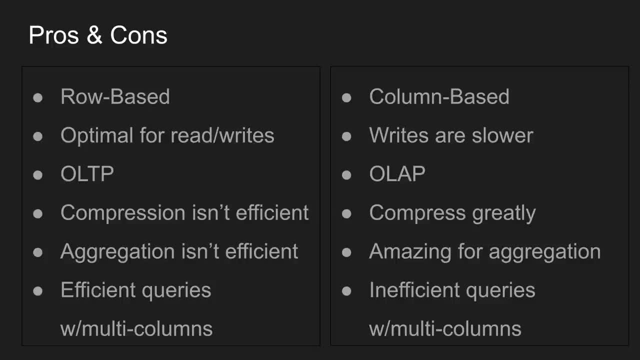 you can pick a date table and you store this table as column store and you can pick another table and store it as row store. you can swizzle the database engine right based on that. you can just change your database engine for every table based on the needs. if you have a table that only get queried. 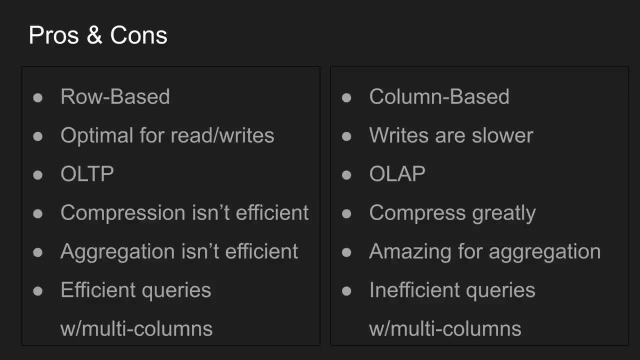 make it column, for example, right if you're doing a lot of analytics on it. make it a column right if you're doing a lot of writes and probably you want to make it a row store right and think about all of this stuff like you cannot, for example, join a row based store, call a table.